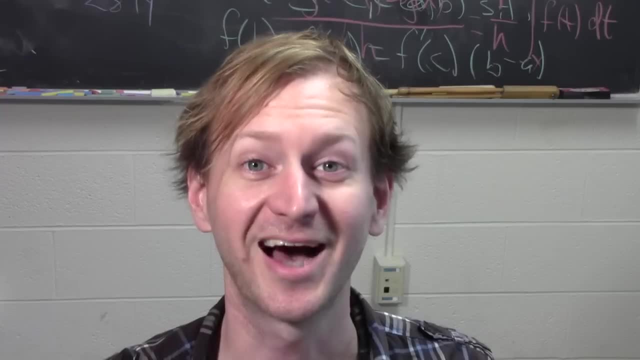 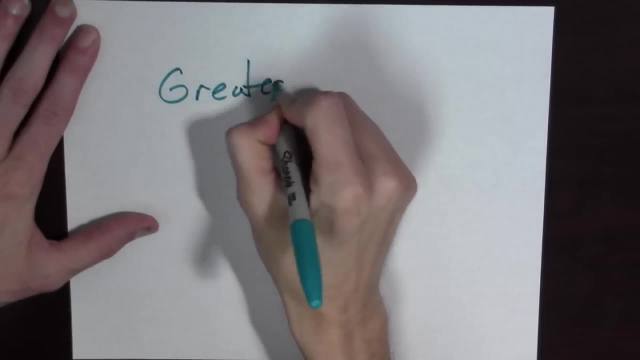 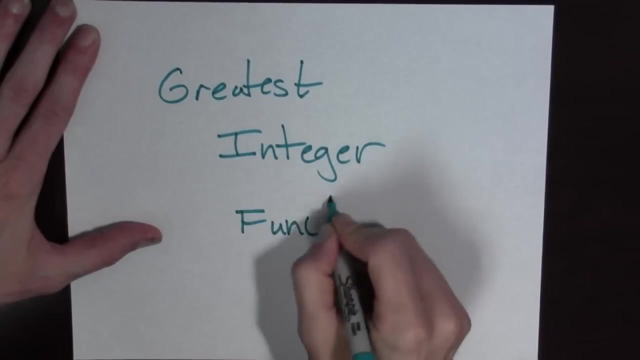 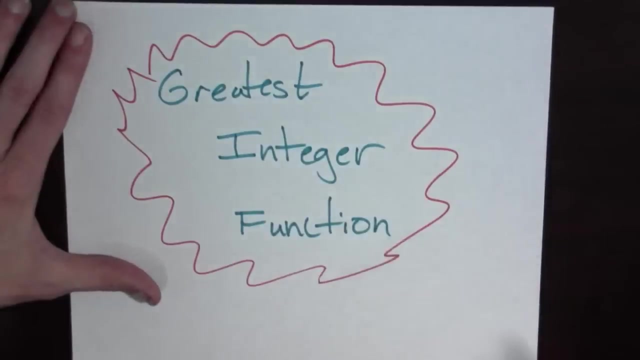 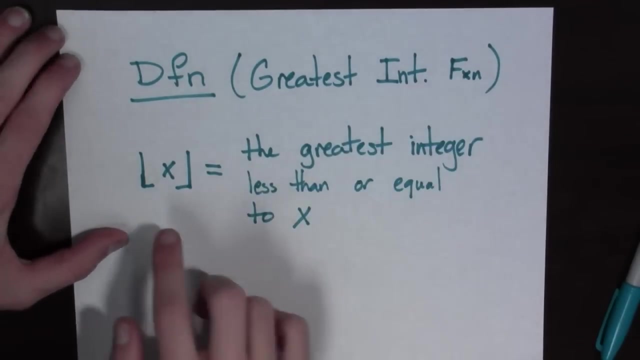 Hi there, One of my favorite functions is the greatest integer function. What's this? You've never heard of the greatest integer function. So the greatest integer function, which we denote by these funny bracket thingies, takes a real number, x, and outputs the greatest integer that's less than or equal to x. 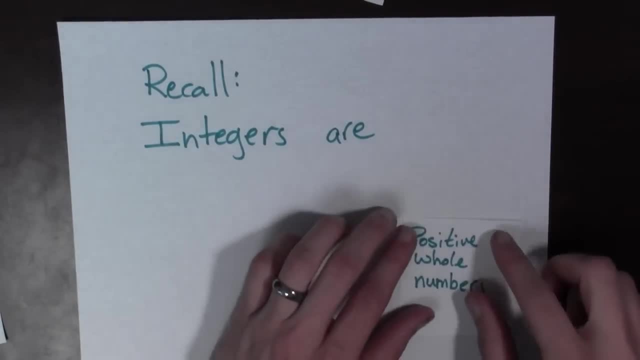 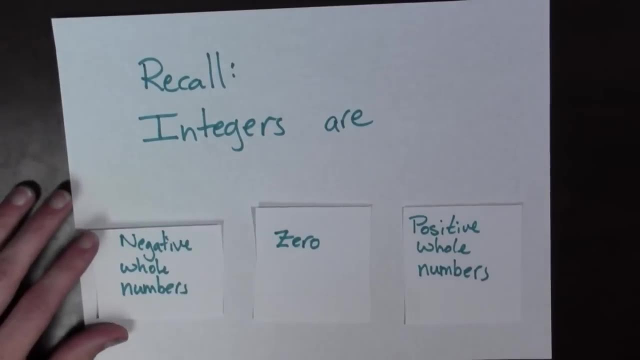 Recall that the integers are the set containing the positive whole numbers- 0, and the negative whole numbers. And if you want an example of this, well, positive whole numbers are numbers like 1,, 2,, 3,, 4,, 5,, 6,, 7, and so on. 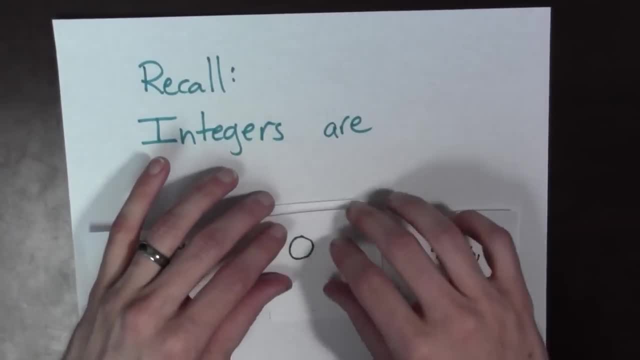 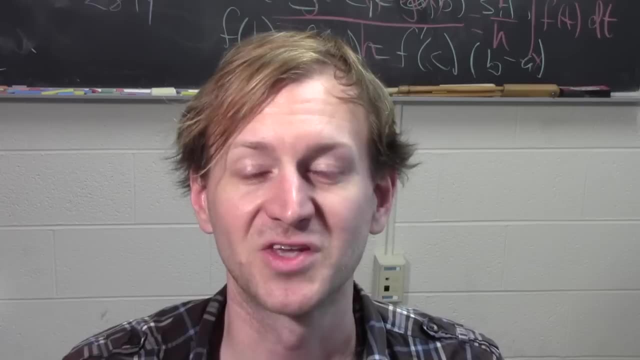 0.. Well, we all know what 0 is. 0 is just 0. And negative whole numbers are numbers like negative 1, negative 2, negative 3, negative 4, and so on. So any function from the real numbers to the real numbers can be plotted. 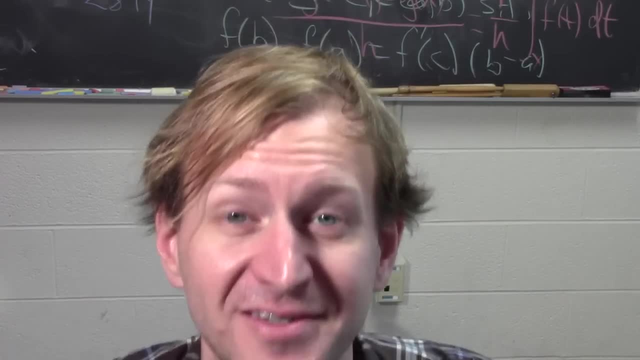 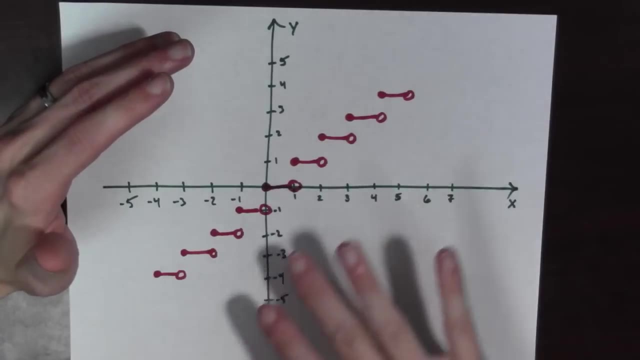 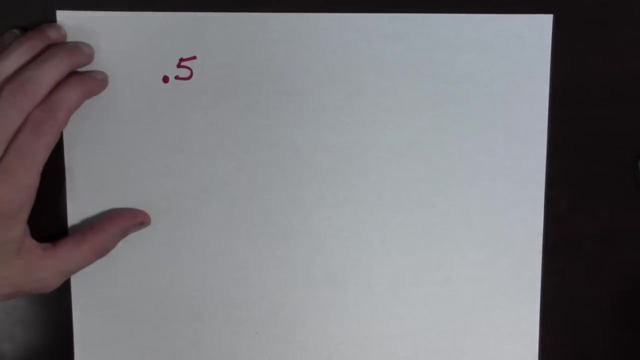 Let's go ahead and plot the greatest integer function. So here we have a plot of the greatest integer function. Let's see if we can explain why the plot looks the way it does. Consider the number 0.5.. When we evaluate the greatest integer function at 0.5, we get 0.. 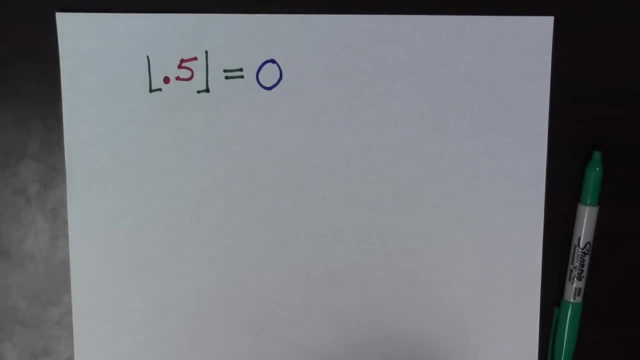 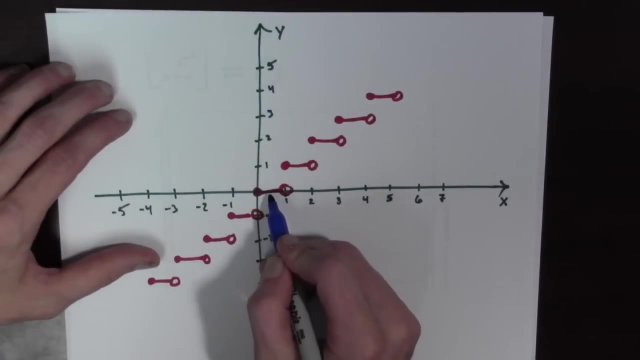 Because 0 is the greatest integer, that's less than or equal to 0.5.. Let's look at the graph again So see 0.5 has a y value of 0. So the greatest integer sends it to 0.. 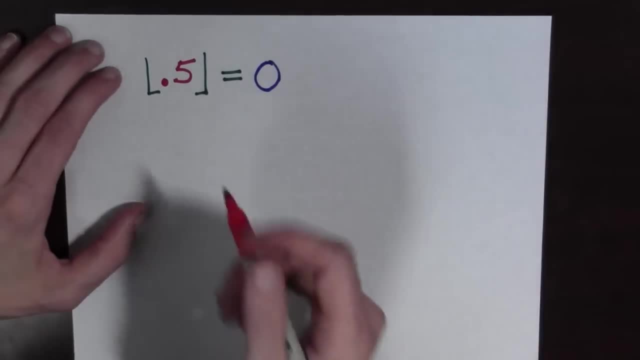 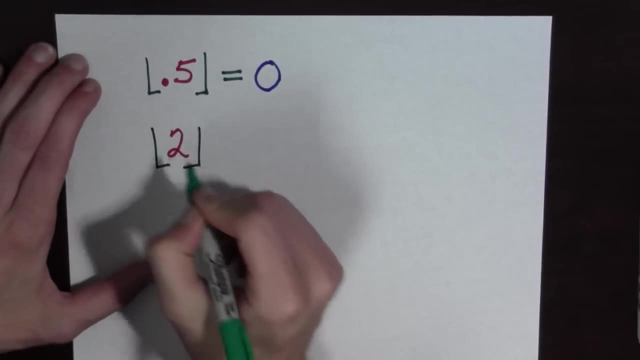 Let's do another example. So now, instead of 0.5, let's look at 2.. What's the greatest integer that's less than or equal to 2?? So that's what this symbol means. It means you find the greatest integer that's less than or equal to 2..